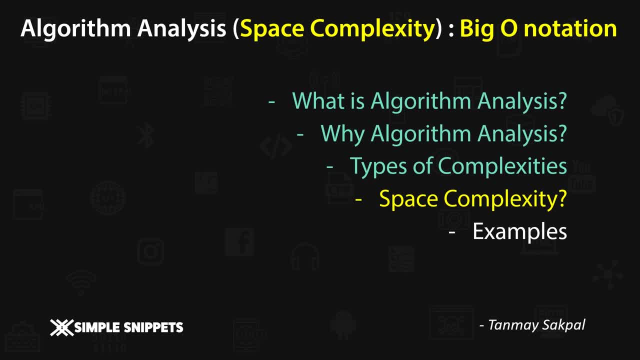 understand. So, with that being said, enough of the introduction, let's just jump into it Now. a quick recap: we already know. what is Algorithm Analysis? why is Algorithm Analysis needed? types of complexity. what is Big O Notation? what is Big O Notation? what is Big O Notation? 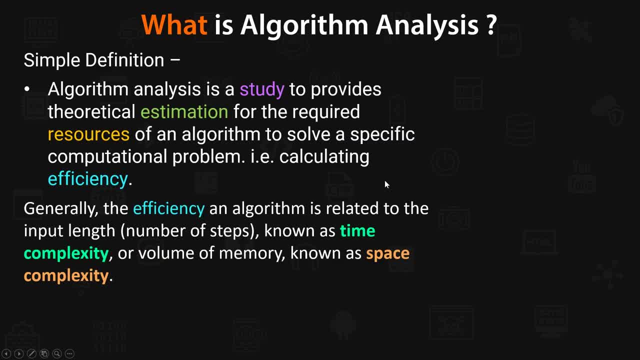 what is multiple complexity? So just scrolling through the slides, you guys can pause the screen and you know, read the theory. it's pretty understandable. What is Algorithm Analysis? it's the study and theoretical estimations of the resources of an Algorithm. that is. 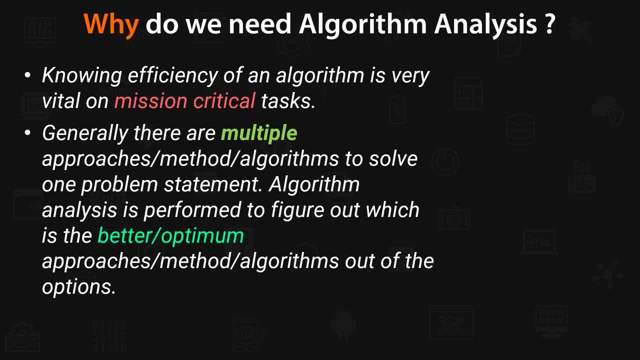 the time and space it requires. Then, moving on, why do we need Algorithm Analysis? because we want to estimate the time and space. Because there are certain times we have some mission critical tasks wherein the time and space matters a lot. So we've discussed this previously. 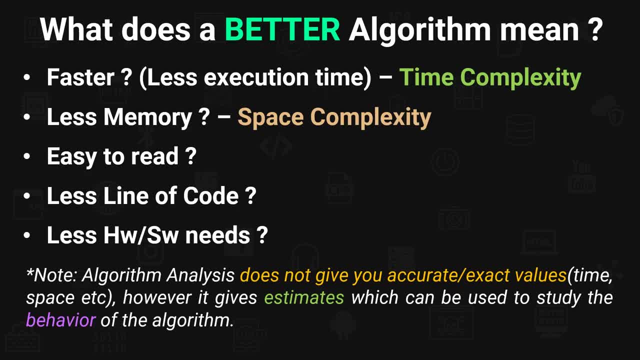 previously, so I'm just quickly going through the slides. so what does a better algorithm mean in reality? well, the two major factors are: how fast is your algorithm which is dealing with the time, so that's the time complexity, and how much memory is your algorithm occupying, which is lesser? the 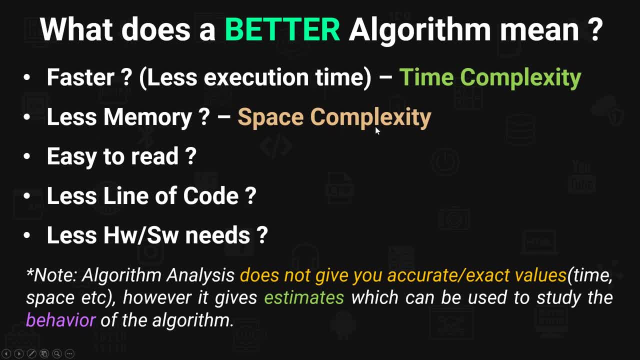 memory, the better the algorithm. so that's the space complexity. okay, so we are going to focus on space complexity. then there are other parameters also which are not really that important. the first two are the more important ones and moving ahead to the real topic, that is, space complexity. now 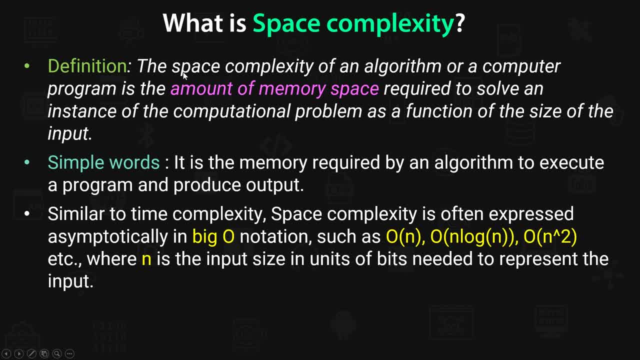 the formal definition of space complexity is as follows. let's cover a little bit of theory before we actually jump into the examples now. the space complexity of an algorithm or a computer program is the amount of memory space required to solve an instance of the computational problem as a. 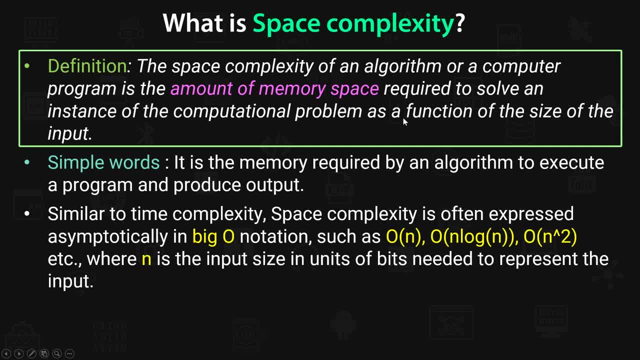 function of the size of the input. now this sounds like a little tricky and little difficult definition, because it's directly from wikipedia and they don't make it easy right, so put it in simple words: it is the memory required by an algorithm to execute a program and produce output. that's the very simple definition. so we are dealing with space, which. 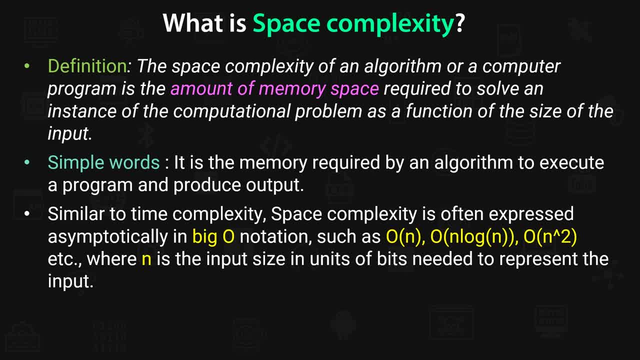 means we are dealing with memory, because every algorithm which we write as a code and run in a computer, it is going to run in your main memory and it is going to occupy some memory. so we want to estimate how much memory is that algorithm going to occupy and the reason we want to make. 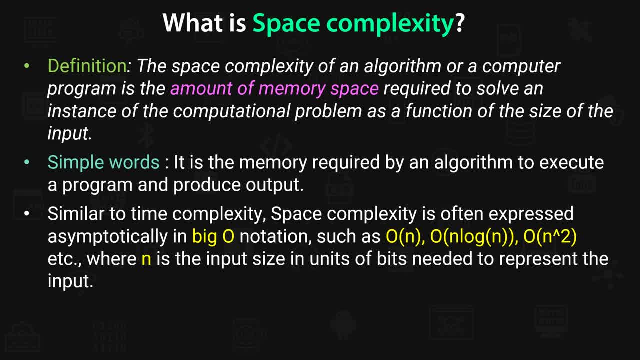 estimations is because we already know that when we want to solve a particular problem, generally we have multiple approaches, multiple algorithms to solve the same problem. for example, if you want to solve in an array, we have two simple algorithms, which is linear search and binary search. so there, 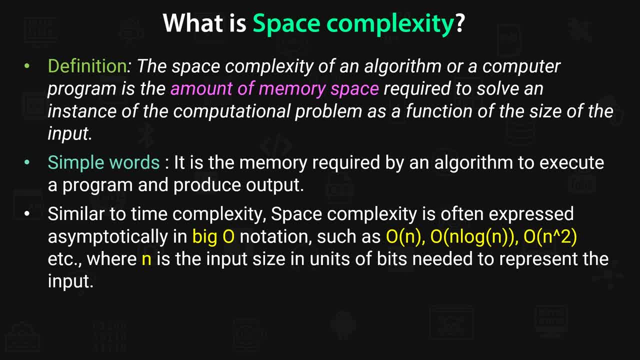 are two options. similarly, when you want to perform sorting, we have different sorting algorithms, which means we have different options and each of them have their pros and cons, and that's why we want to make an estimate about algorithms and how much space they are gonna occupy. so this video we are 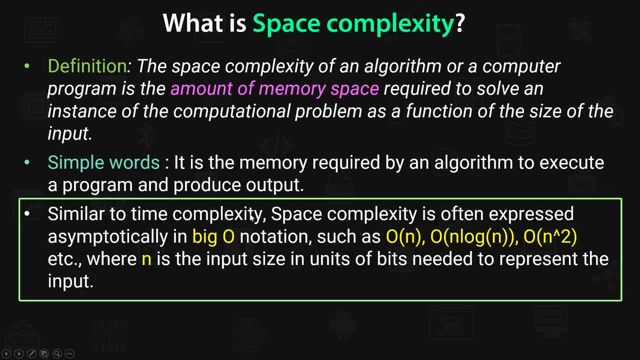 only going to talk about space and not time now. similar to time complexity, space complexity is often expressed in asymptotically in the big O notation. so just like we have big O notation for n big of n square and so on and so forth, similarly space complexity also is denoted by big O notation. 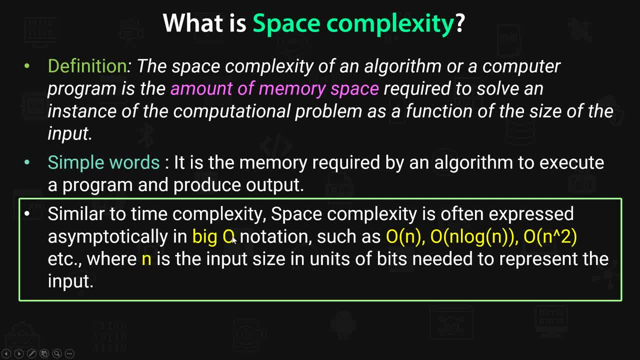 only because big O notation is just a mathematical notation which gives us the relation of how the space changes depending upon the input size. so as the input size increases, let's say, the size of the array or a data structure is phi, so phi items are there in a data structure, the space occupied, let's. 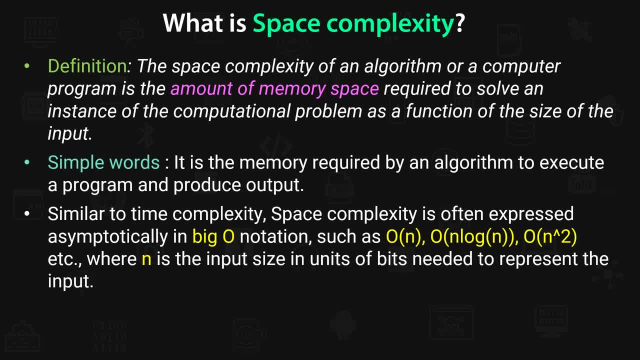 say, is 10 mb. and now, if I double the size, is it becoming 20 or is it becoming 40, or is it becoming exponentially growing? that is the you know. that is what we are actually tracking over here. so this big O notation just gives us the behavior right. so we have the same big O notation in space complexity. 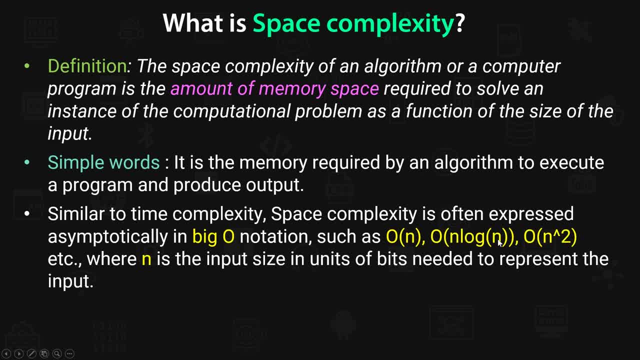 also like O of n, O of n log, n, O of n square. now these are all functions which can be shown on a graph. mathematically also, we've seen in the time complexity video where n is the input size. now things get a little tricky, as I mentioned in space complexity, because there is a little bit of 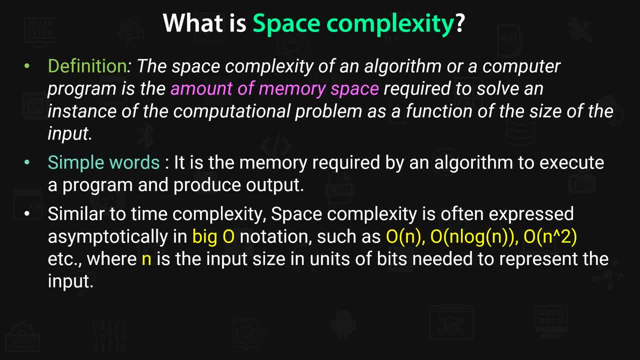 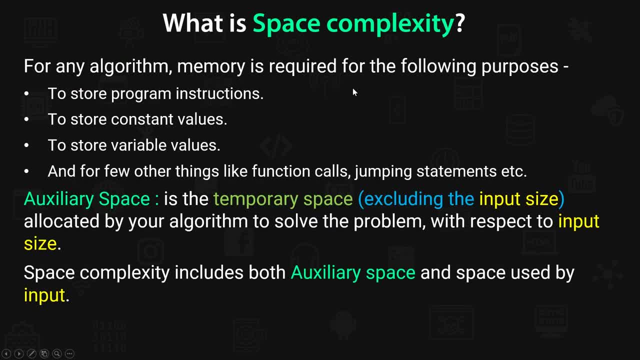 misconception when it comes to calculating space complexity, because there are two ways to look at space complexity. so let's talk about that now. for any algorithm, a memory is required for the following purposes: obviously to store the program instructions, so every statement would be actually an instruction. we need to store it somewhere. to store the constant values, to store the variables. 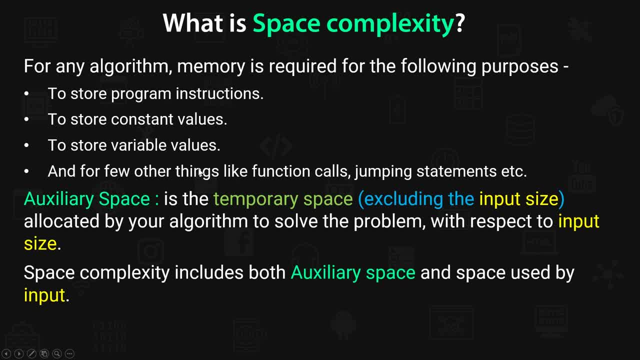 that we create. and then there are few other things like function calls and jumping statements. now these functions calls are important to keep a track of because what happens is when you write big algorithms, one function calls other function, the other function might call multiple other functions, so we need to keep a track of who is calling whom right. so there is a call stack concept. 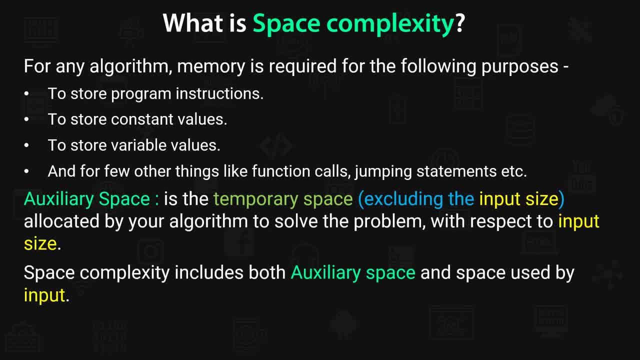 which is basically a stack which is provided by the system. we don't have a track of it which keeps a track of all these function calls- who is calling whom? we'll talk more about that when we take the example, so stay tuned for that. don't skip this video. watch this video till the end, so that's. 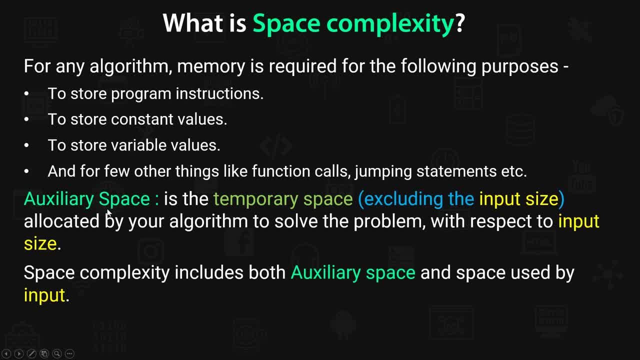 where the auxiliary space comes into picture. so what is this auxiliary space? so the auxiliary space is the temporary space excluding the input size, excluding the actual data structure. okay, that we are working on. so let's say you are performing sorting on an array of size, phi, so that input size of that. 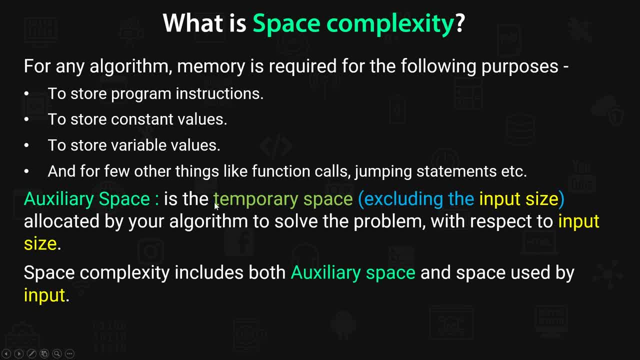 array is size, phi, right, so excluding that whatever extra space is required by the algorithm can be considered as auxiliary space. okay, so that's why auxiliary space is the temporary space excluding the input size allocated by algorithm to solve the problem with respect to the input size. now, when it comes to calculating the space complexity as a whole, 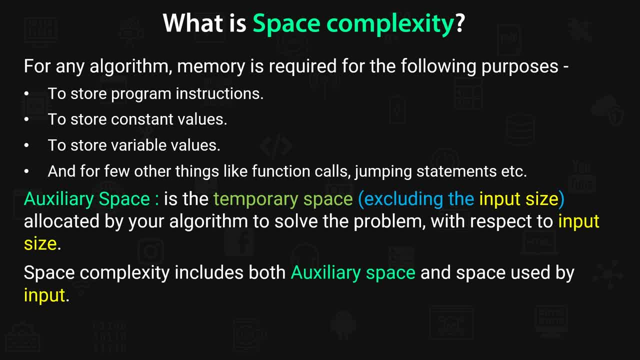 it includes both auxiliary space and space used by the input. so it's basically auxiliary space space plus the space used by the input. Now, this is one way to look at space complexity. However, sometimes what happens is we do not consider this as the actual measure. We only 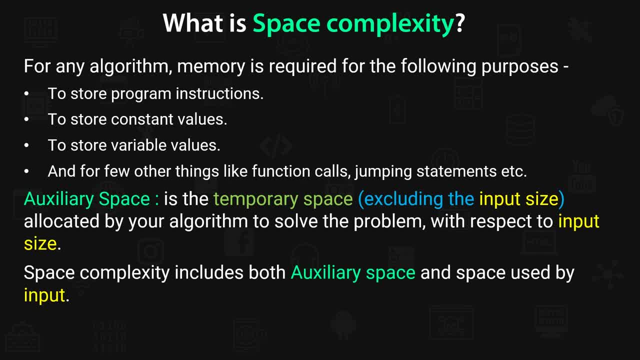 look at the auxiliary space Now. if it is getting a little confusing, don't worry, I'm going to solve this doubt and solve this confusion once and for all. Let's actually take an example and let's jump to the digital blackboard. Let's see what happens behind the scenes by 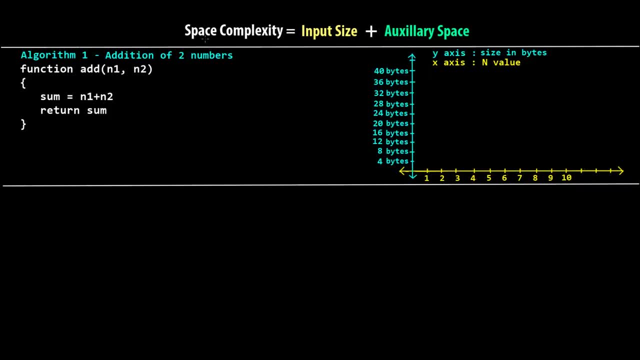 taking different algorithm examples. Okay, so, as I mentioned, space complexity as a whole is equal to input size plus the extra auxiliary space. right, We just talked about it theoretically, So let's take an algorithm over here which is basically a very simple algorithm of addition. 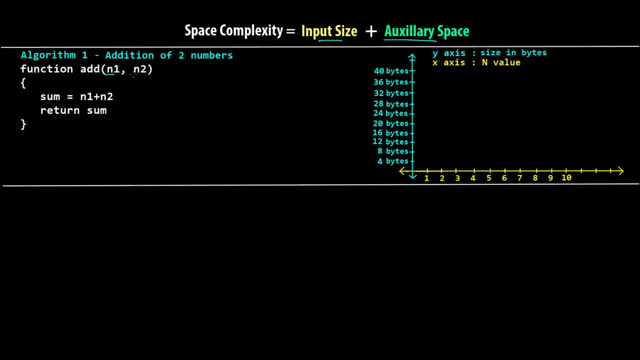 of two numbers. So this is the function. it takes n1- n2.. So n1 and n2 are two variables, Let's say they are integer variables. you create a third variable, sum. you store the addition in that some variable and you return that from the function. Okay, very basic. 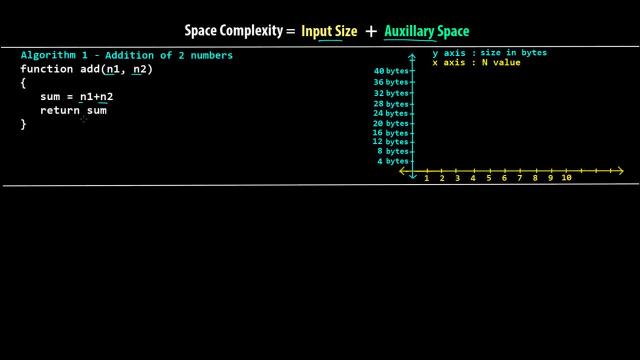 Now if you want to actually estimate the size that this function would take, you can easily try to estimate it by just by calculating the size these variables will take, right? So let's say n1 is an integer variable And assuming that integer variable takes four, 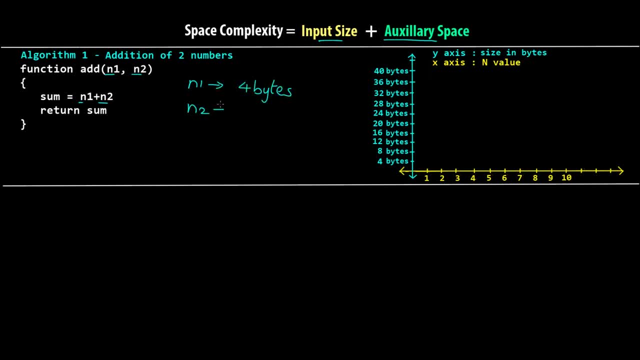 bytes. n1 will take four bytes. n2 will take four bytes. this sum variable will take, let's say, four bytes again. So this is all the memory that all the variables are going to take Now. apart from that, obviously there will be some overhead, which will be the auxiliary. 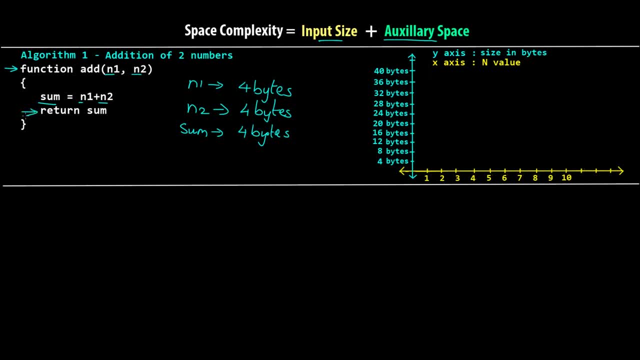 space, which is these instructions: this function: call this return statement. this function- let's assume that it is going to take some constant space- only because obviously we are not increasing the number of statements, these statements are going to be as it is. 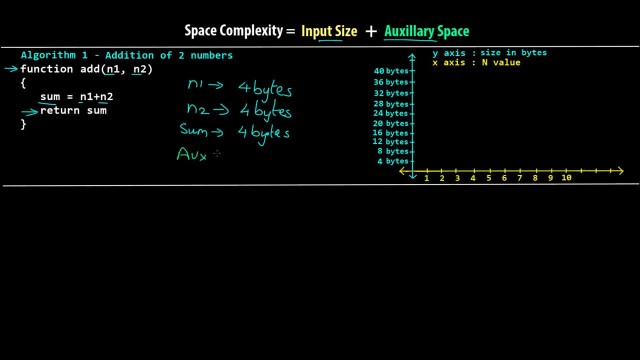 So let's assume that the auxiliary space- so I'll say aux SP, is four bytes. So if you do a total, the estimated total, obviously this is the estimated total. this is not the actual total- is going to be four plus four plus four plus four, which is 16 bytes. Okay, 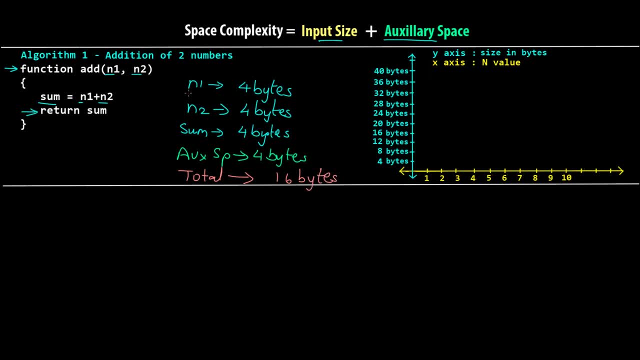 Now, no matter what is n1 and n2, when I say what is n1 and n2, which is n1 and n2, which is the value, so let's say I'm passing five and five, it's going to be some, some is going. 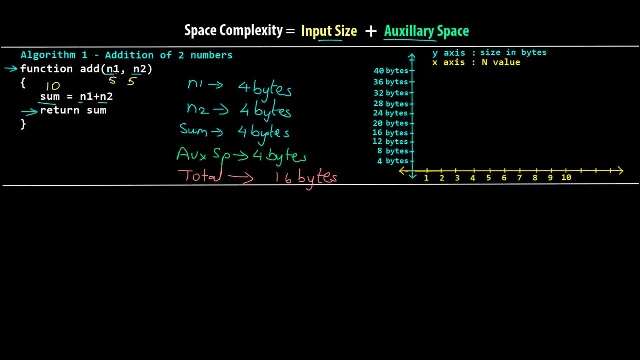 to be 10.. So even then it is going to occupy 16 bytes, because that integer variable is going to occupy four bytes only in the memory. Let's say, if I pass 110 and 90, so the total is going to be 200. But still n1 and n2, that is, these two variables are obviously. 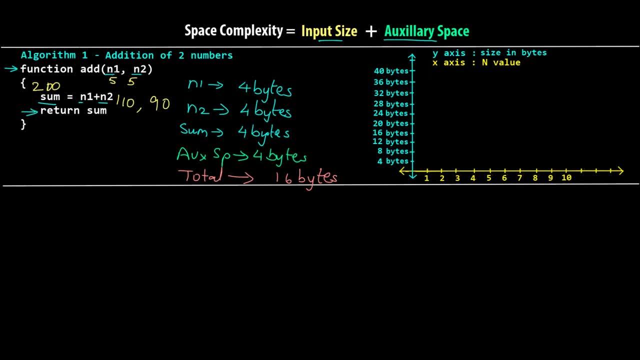 going to occupy only four bytes. even though I increase the actual value which is stored inside these variables, the memory that they're going to occupy is always going to be constant, right? So no matter what value I pass over here, the total is approximately going to: 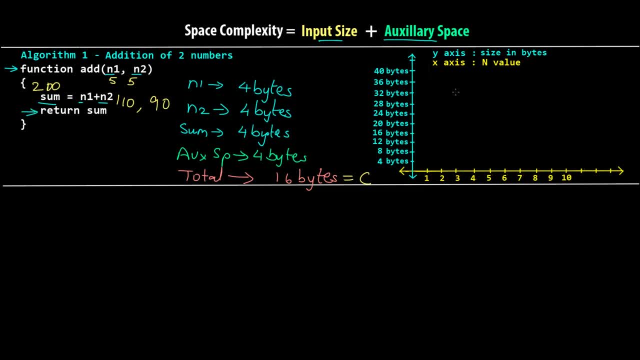 be 16 bytes only, which is actually a constant value. So if you track it on a graph, y being the size in bytes that this program is occupying and the yellow axis is actually the size, that is the input size. over here, the input size is not changing. the input size is actually. 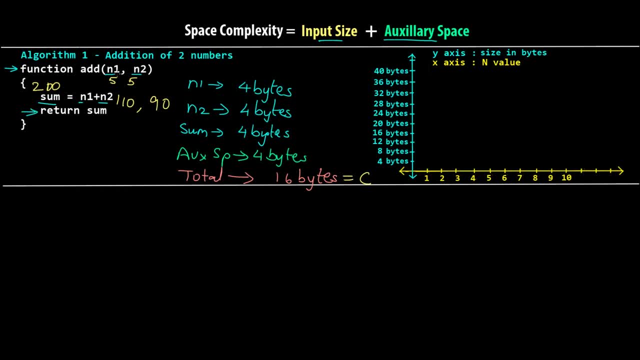 going to be a constant value And we are having two variables, And let's assume that we're just having two variables. So, no matter what, we are constantly at 16 bytes only. So the graph would look something like this: So, no matter what value. 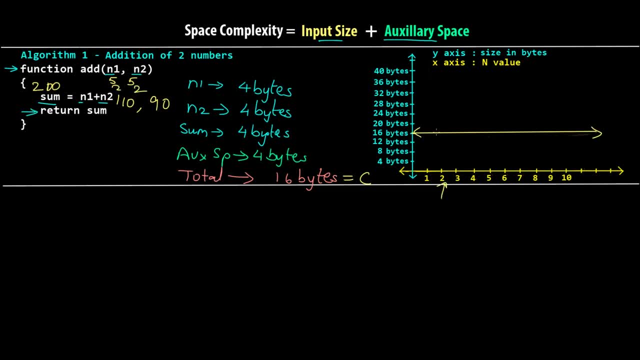 you pass, let's say you pass- two and two over here. two and two, it is still going to occupy 16 bytes. if you pass 10 and 10, that is n1 and n2 is 10 and 10, even then it is obviously. 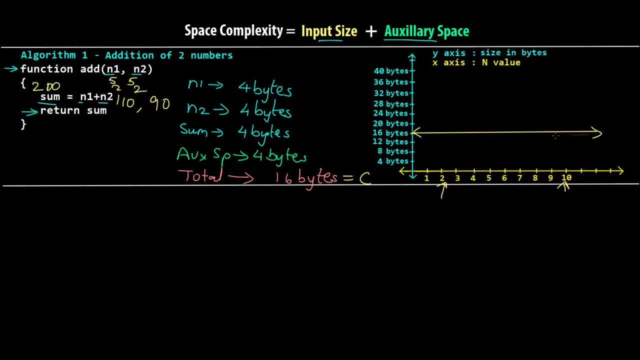 going to occupy 16 bytes only, So you can see it is a straight line, which means it is a constant space. you can say that it is constant right Now the way we represent constant space or constant, you know, constant behavior. 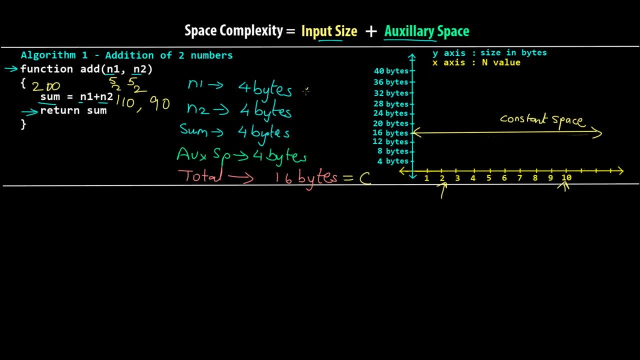 Is by big O of one. So the final result would be O of one, because it is a constant, no matter what the input, or whatever value you're giving of the input. the size that this program is occupying is more or less going to be 16 bytes only. Hence this algorithm can be considered. 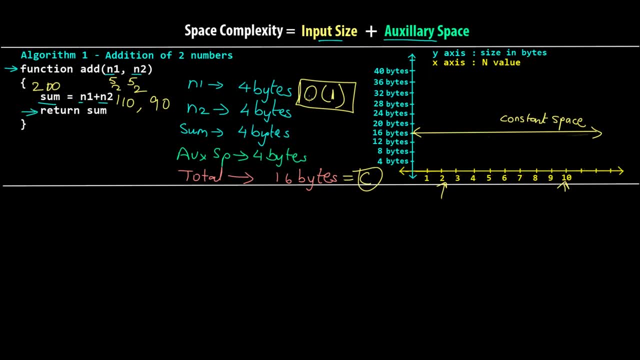 as a O of one space complexity algorithm. So I hope you're understanding this. If you've seen the time complexity videos, this should be easy to understand. Let's take another algorithm to better understand this. This time, the algorithm is some of all elements in an area, So we are passing the area. we 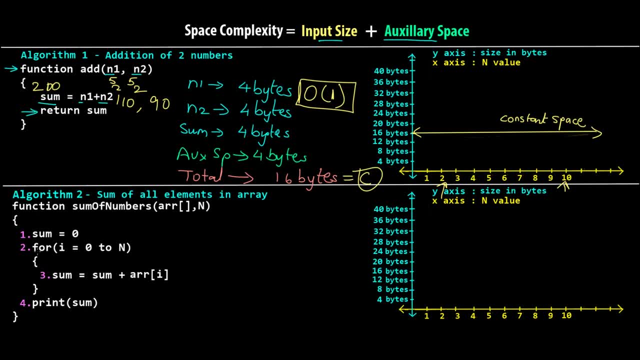 are passing the size of the area, we are declaring a some variable and we are using a loop to iterate through all the elements inside the area. So zero to n, so n is the size right. So from zero till the size, and we are seeing some is equal to some plus err of I. So this 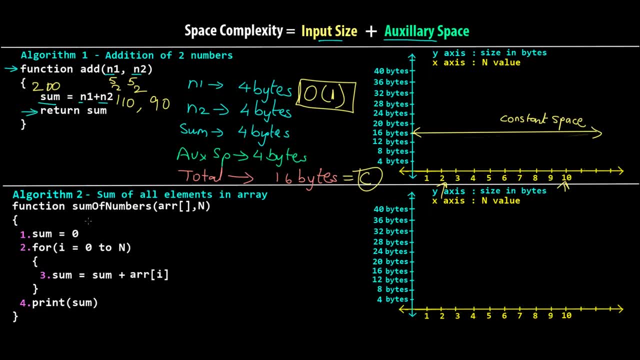 is that iterator And then, ultimately, we are printing it. Now let's analyze this. we have an array which is of variable size of n. So if it is an integer array- let's assume it is an integer array- the size of this array, that is, arr, is going to be equal to n into 4 bytes. 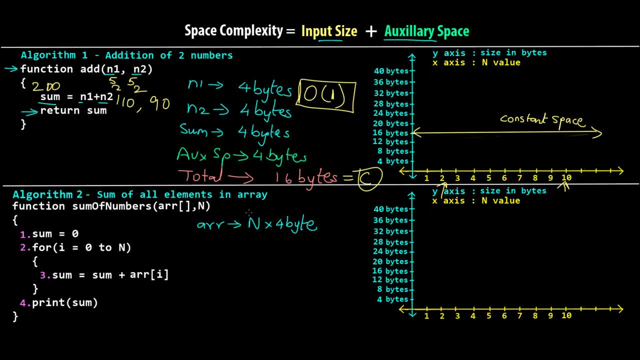 right. so if the size of the array is 5, so 5 into 4, 20 bytes of space is going to be taking into the memory. if it is 10, so 10 into 4, 40 bytes. so n is the variable over here. so n can keep on. 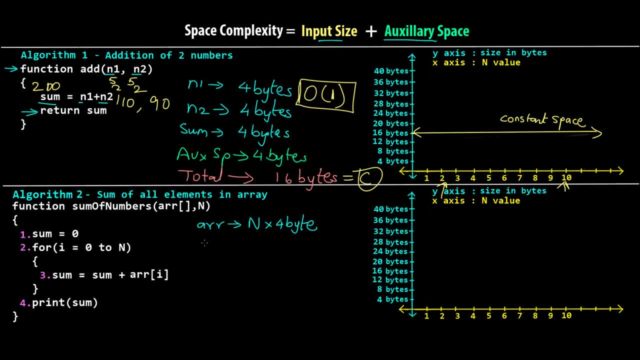 changing. it is not a constant. now other things are pretty much going to be constant because some variable is going to take 4 bytes. when we initialize the for loop, we are creating iterator i. so this i variable again is an integer. it's going to take 4 bytes and this is for the variables. 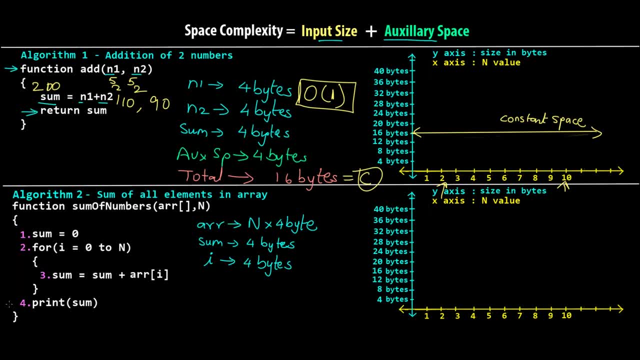 the other things like initialization of the for loop, the printing statement, the function call. these are all auxiliary spaces. so the auxiliary space, let's assume it, takes 4 bytes. okay, now, if you sum all this up this time, the total, which is actually the space complexity that 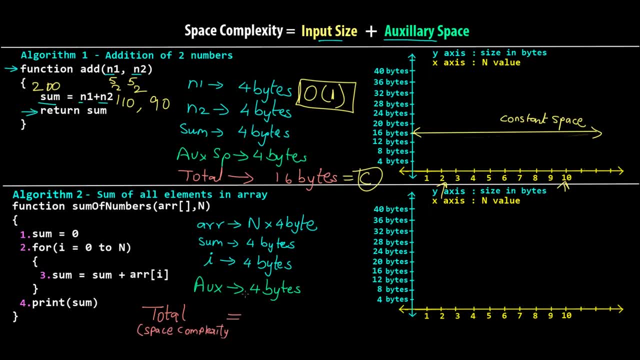 we are calculating can be given as n into 4, so that is 4n plus 4 plus 4 plus 4. so these two are the variables and this is the auxiliary space. so we have 12 bytes. so now you can see that we have one variable over here and this variable will keep on changing depending upon 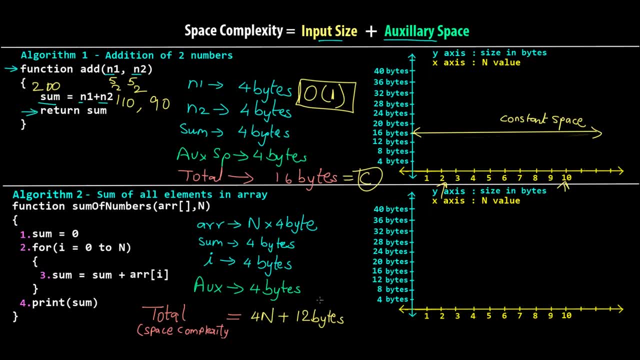 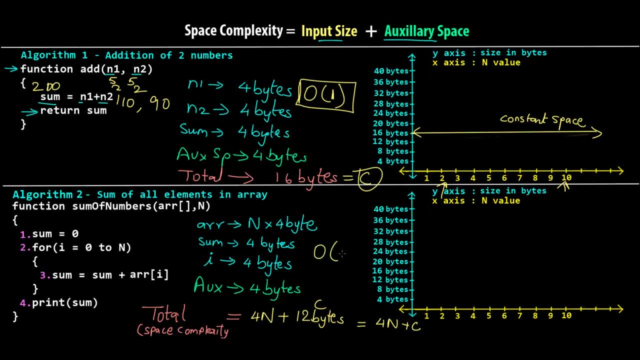 constant values, we are ultimately left out with o of n, and this is the space complexity for this function. but this is the overall space complexity. we are not looking at just the auxiliary space over here. and if you see the graph of this algorithm, depending upon the size, 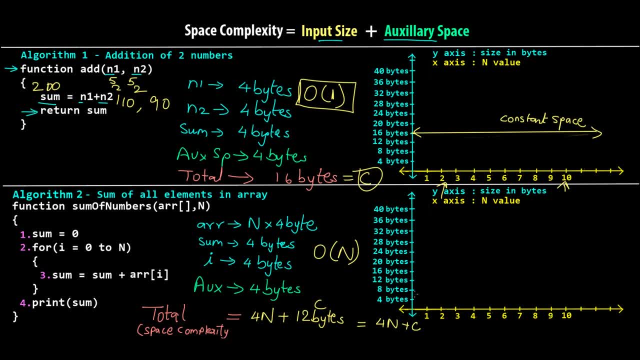 of the array. the graph will also go on increasing. so for n equals to 1, 4 bytes will be allocated for the array, and then obviously plus 12 bytes, right? so 4 plus 12 will be 18 bytes if n equals to 2. so if i substitute 2 over here, 4, 2s are 8, so 8 bytes plus 12 bytes. 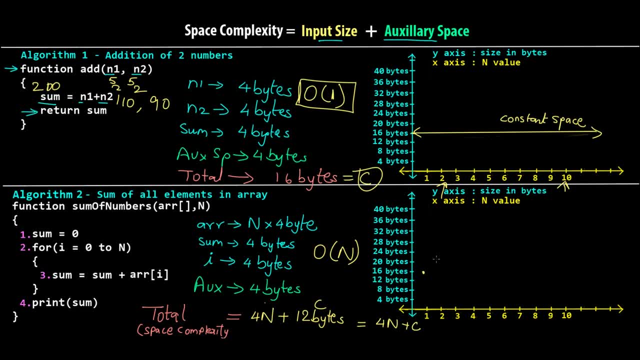 so 8 plus 12 is 20 bytes, which is somewhere over here now. if n becomes 3, if i substitute 3 over here, 4, 3s are 12. 12 plus 12 is 24 bytes, which is somewhere over here now, if you see. 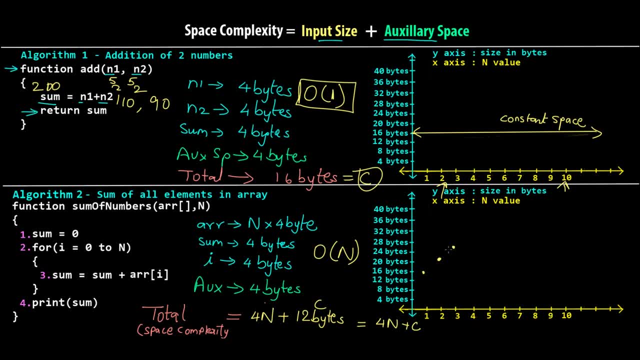 there is a pattern going on: with every n that is incrementing, 4 bytes are being increased, so the next would be 28 somewhere over here. then we have 32, and so on and so forth. so if you just plot this line on the graph, it would look something like this: 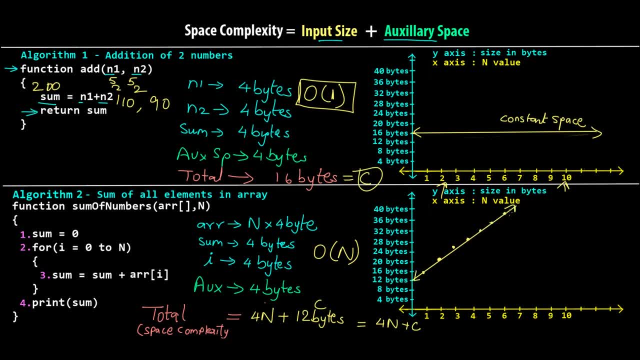 so it would go increase, go on increasing in 4 byte sizes. so this is called as linear space complexity. okay, so i hope you are understanding. but one thing to remember is we are calculating space complexity with this equation, or with this formula, which is input size plus auxiliary. 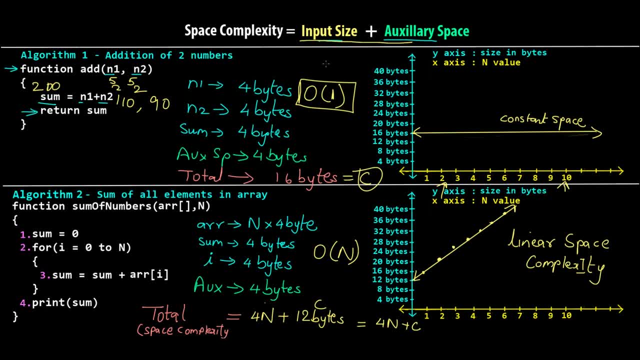 space. now, as i mentioned a lot of times, what happens is the input size is not considered when calculating space complexity. so if you are wondering why is that, it's because when you are writing an algorithm on a particular data structure, if you consider the size of the data structure, then that space complexity will always be there you want to calculate. 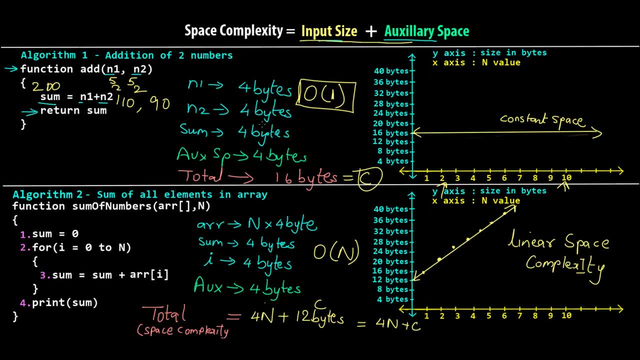 the space complexity of the algorithm and not the input that you are providing to the algorithm, because you want to track how much space is taken given a particular input size. so if you calculate the space of the input size also along with it, that basically rules out the purpose of actually doing or calculating the space complexity. so if you calculate the 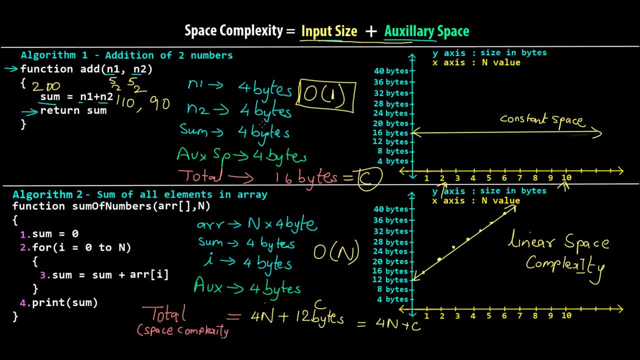 space complexity itself. now, if it is not still making sense, let's actually take two more examples. so so far, so good. i hope you understood what is space complexity and how you calculate space complexity using this formula, which, which is input size plus auxiliary space. now there is another way, as i mentioned, wherein we are only considering auxiliary. 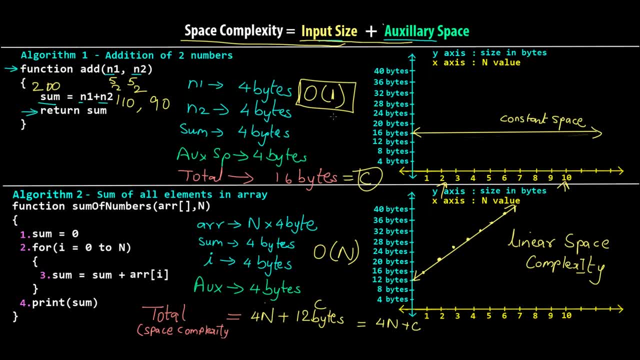 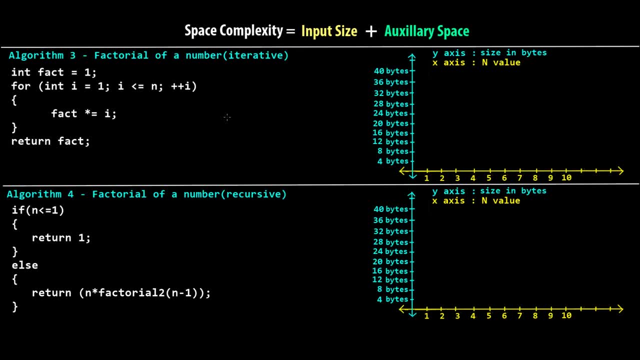 space. and why is that? so? we'll see that in this. further two examples. now, generally, when we look at algorithms, we can broadly classify them into iterative or recursive. now, iterative is when we perform multiple activities over and over again, and recursive is when we are using the function to call itself, which is basically the concept of recursion. now we've 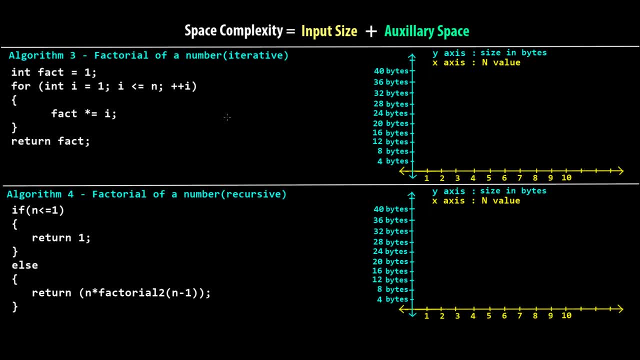 already talked about recursion in the previous tutorial when we did the merge sort in this series. i have a separate dedicated video also which explains what exactly is recursion and how it works behind the scenes, so i'll drop those links. if you have even one percent confusion about recursion, please watch that video. that is very, very important and very, very easy. 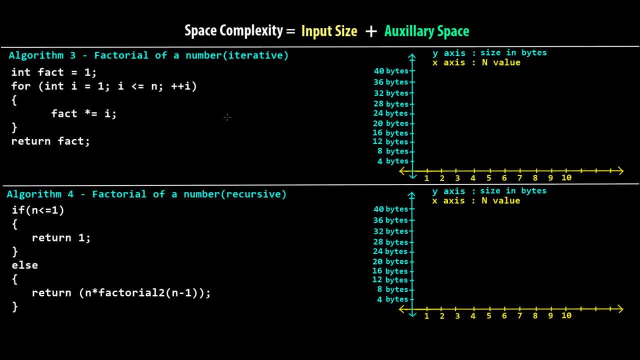 and detailed to understand and then come back over here. but, as i mentioned, generally, we can broadly classify them into two types, that is, iterative and recursive. now, if you see algorithm 3 and algorithm 4, both are solving the same problem, that is the problem. statement is same, that is, we want to calculate factorial of a number. 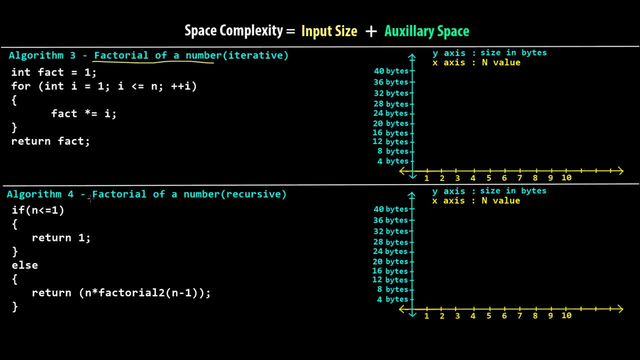 but here we are using the iterative method. algorithm 4 again says factorial of a number, but we are using the recursive method. now let's actually calculate the space complexity over here using this formula, and then we'll also only calculate the auxiliary space complexity also okay. so here we are declaring a variable. in fact, then we are using the loop. we are going from i to 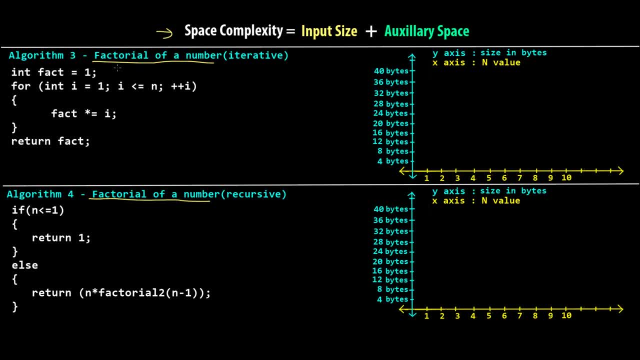 n. so the n is basically the number that we want to calculate the factorial of. okay, so n would be something that is going to be coming from the user. so let's say n equals to phi. so if i say phi, the factorial of phi is going to be 5 into 4, into 3, into 2, into 1. so i hope you know what is. 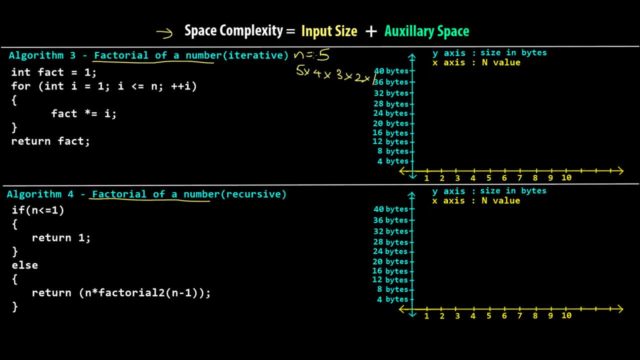 factorial and how to calculate that mathematically. when i say n equals to 5, this is what should happen in the algorithm. so let's say i am saying n equals to 5 over here. okay, so i'm declaring a variable fact. i'm going from int. i equals to 1, i less than equal to n. 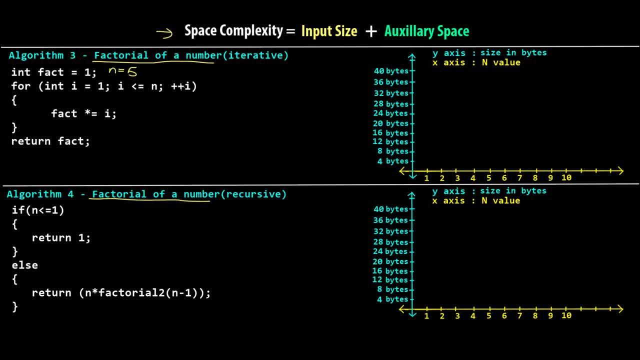 so n is phi. so i'm going to go till phi and then i plus plus or plus plus i, i'm going to say fact is equal to fact, star i. now this is how factorial is calculated. i have a program also on this separately. if you don't know the logic, just actually type this code in your program and see. 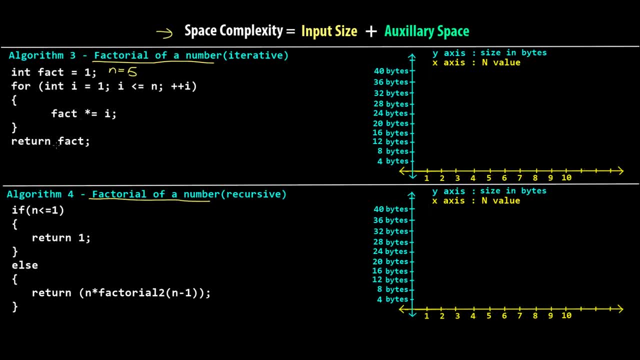 how it goes: step by step. you can try, run it and ultimately you will get the factorial and you can return it from this function. okay, and it will run for five times. so here, if we actually do the space complexity, we have a fact, variable facet which is going to take four bytes, assuming that is. 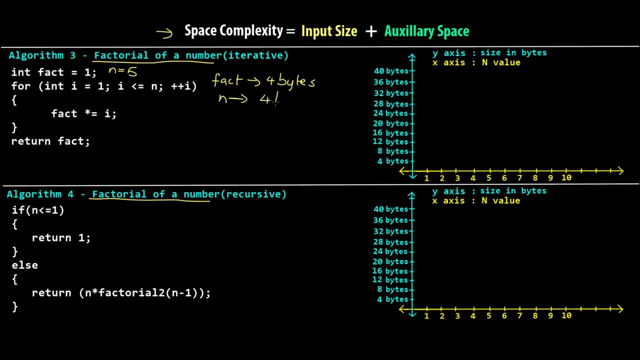 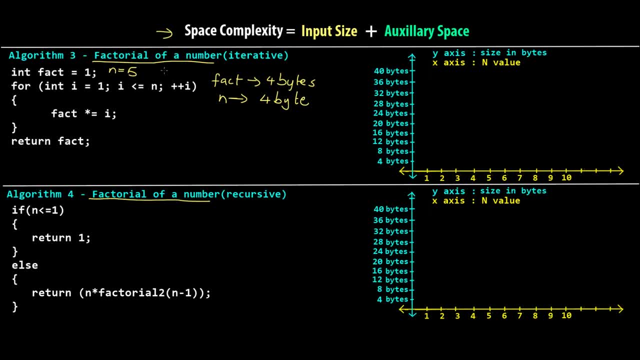 one integer value. so no matter what the integer, be it 5 or 5000 or 10 000 or whatever, it is always going to take 4 bytes. then we have the iterator i inside the for loop, which is going to take 4 bytes. 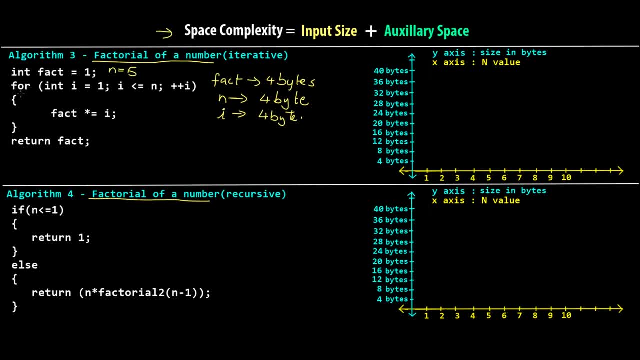 now. now, depending upon what you pass over here- 5, this for loop is going to run for 5 times. if you pass 6, it is going to run for 6 times. so the time complexity over here will vary it, but the size will remain the same because we are not creating additional variables in the loop. we are using the 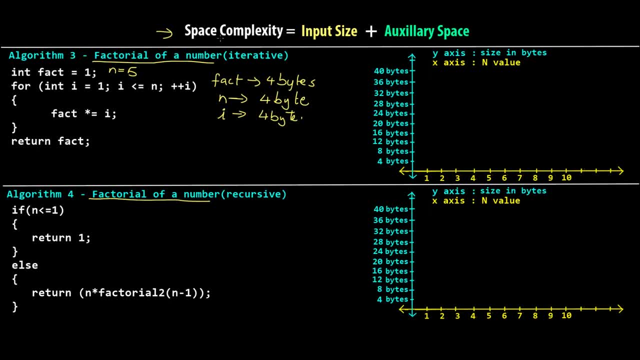 same variables and since we are only interested in the space complexity, the space com, the space will always remain the same, no matter how many times this loop is going to run. the space is always going to be the same because we are not creating more variables in every iteration. we 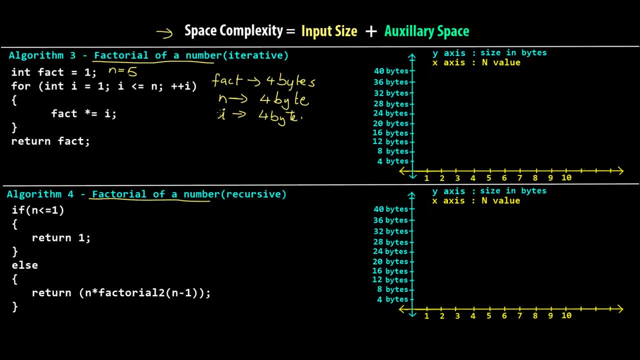 are using the same variable in every iteration, so space obviously going to be the same. and then, ultimately, let's say the auxiliary space, which is used for creating these program statements, running this program statements and storing it somewhere. initializing the for loop using the return statement: all these instructions will also be stored, right. so the auxiliary space. 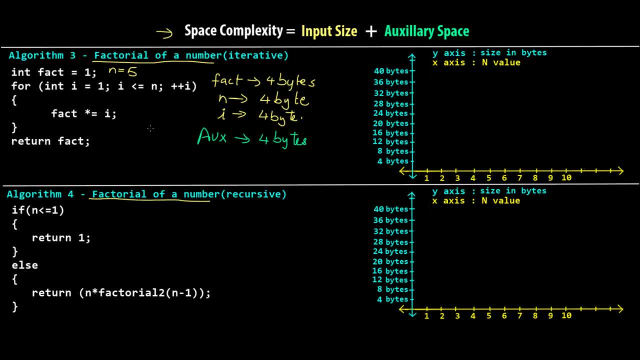 let's say, is 4 bytes. now, in total, if we actually go ahead and use this space complexity formula- i'm going to say s over here- is going to be equal to these: 4 plus 4 plus 4, 12 bytes, plus the auxiliary space, which is again 4 bytes. so this becomes a constant number: 16 bytes. 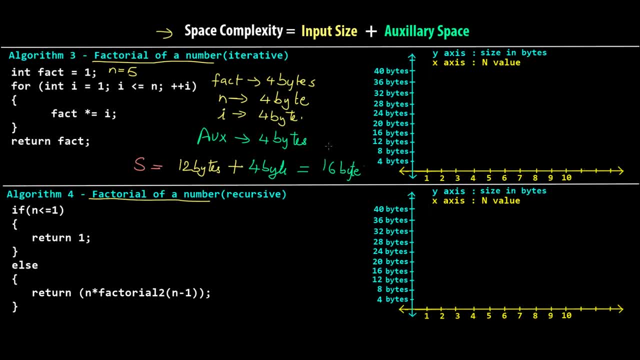 right. so this becomes a 16 byte constant number. so the space complexity over here can be given by big o of one. so whenever we get a constant number and not a variable, we denote it as big o of one. so no matter what the size, the 16 byte is going to be constant. 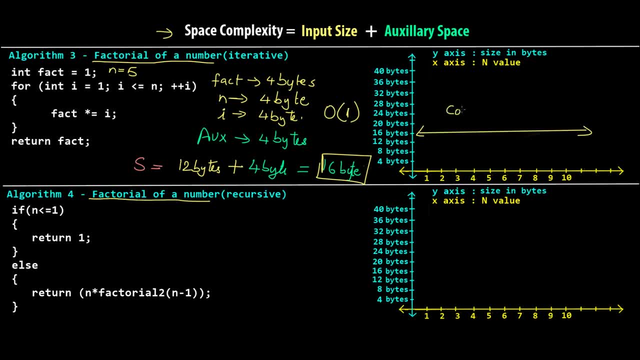 and the graph is pretty much going to look something like this. so this is constant space complexity. now coming to this recursive algorithm. let's see what happens at recursive algorithm now. the algorithm is as follows. let's say n is again equal to 5 and we are passing this in this process. 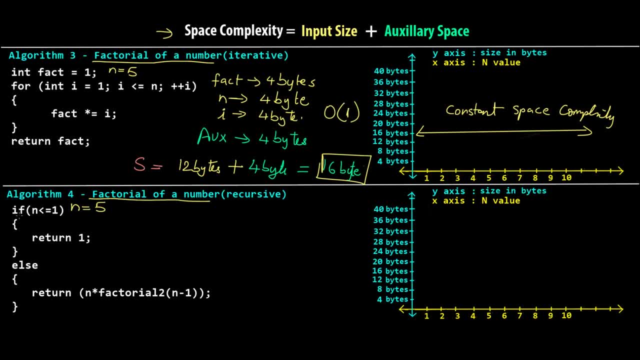 is entirely inside a function. Okay, So first thing we check if n is less than equal to one. if it is less than or equal to one, we have to return one, else we are giving a recursive call and we're seeing return n star factorial, which is actually the name of this function. 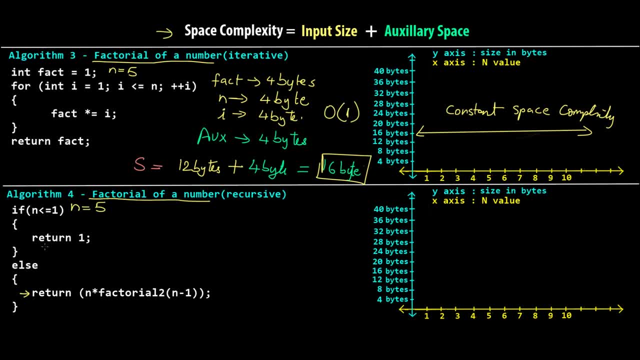 factorial two of n minus one. So we are recursively calling the same function. So factorial two is actually the name of this function. I have not written it over here, But basically, if I would have to show it, it would look something like this: let me just do it, In fact let. 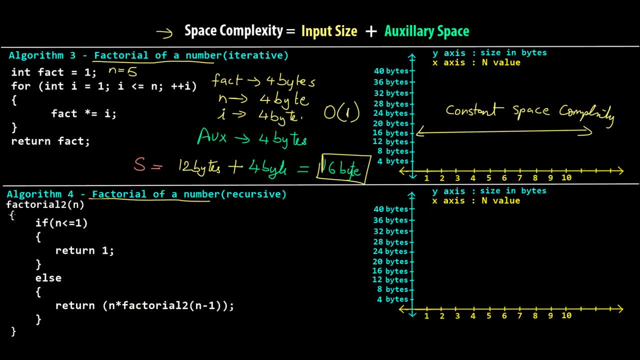 me just put it over here. Okay, so, as you can see, I have modified this and I've added the function name over here. So we are calling the same function, but this time we are saying n minus one. So what will happen? for the first time, we pass phi right. n is equal to phi. 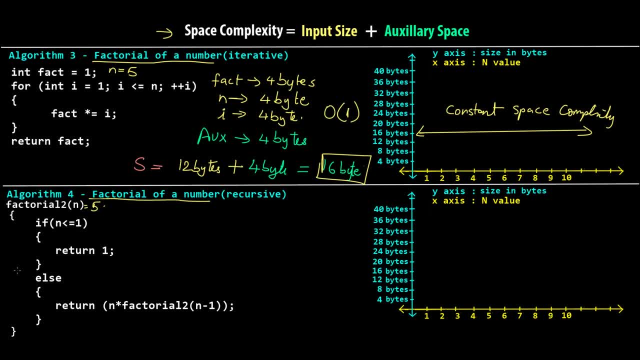 phi is not less than or it is not equal to one. So we'll go in the else part. And now we are giving a call to the same function, factorial two of n minus one, which is phi minus one. So basically, what is happening? First function, we are passing phi, Now we 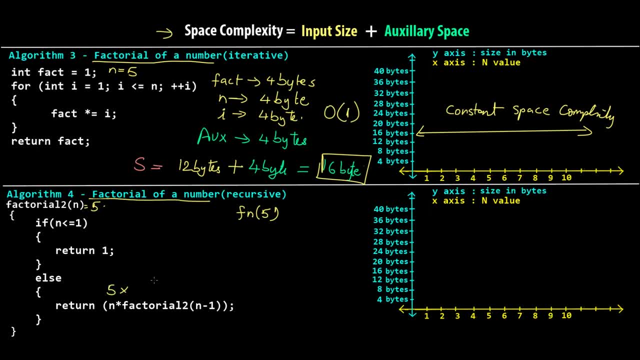 are inside this, we are saying phi into this again, function is called, but this time it is f of n minus one, which is four. So we still don't know what is f of four. we have to call f of four and f of five will be paused. So there is a call stack which is going to 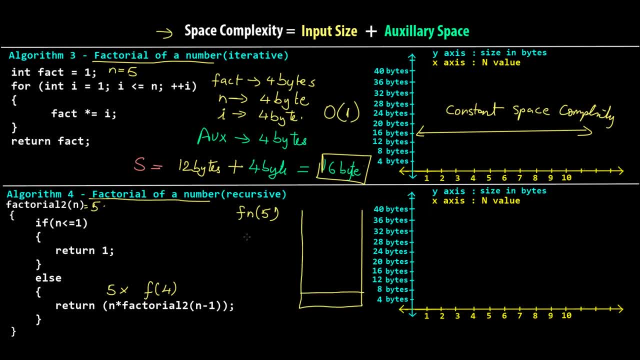 be generated by the system itself, And f of n will actually call f of four. So f of four will be placed in the call stack. we're going to say phi into f of four. Right Now we don't know what is f of four. we're just passing four over here. And now another function. 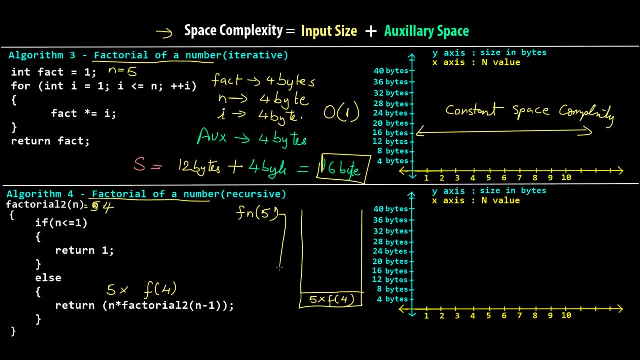 call will be given to the same function. it will become four. So the first function has called this recursively And now we are passing four. is four less than or equal to one? No, So again we'll go in the else part, And now this time it would be n- into again calling. 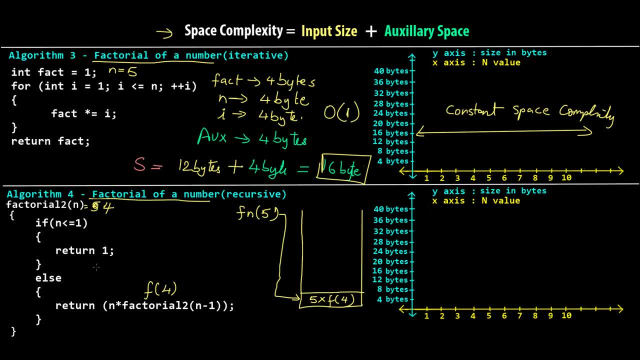 the same function. So this time n is four. So now it would be four into f of four minus one, So it is f of three. So now the call stack will maintain this, because we still have to calculate what is f of three. So we have four into f. 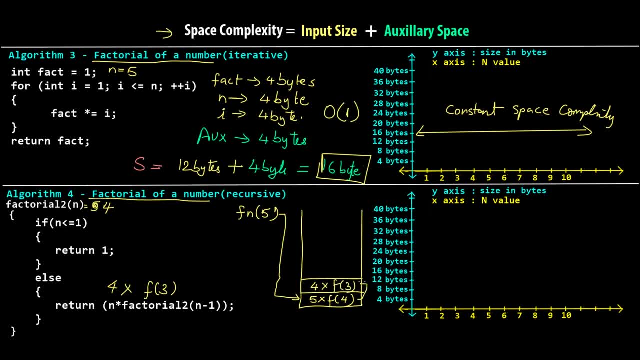 of three. So f of four has basically called f of three. And similarly we will have more calls, So it would be three into f of two. f of two will call f of one, So that would be two into f of one. And when n is going to be equal to one, when n is going to be 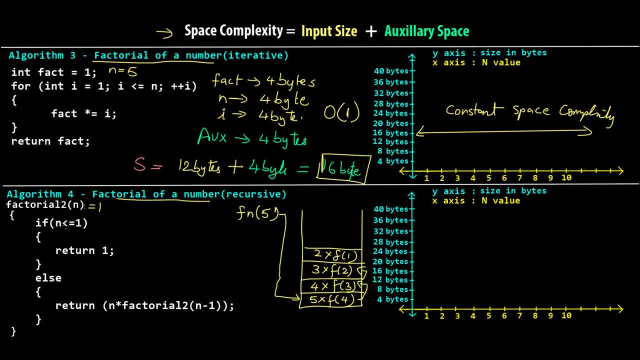 equal to one. that's where this condition will become true. If n is less than or equal to one, it is equal to one. So we're going to return one, So we will not go further from this, and no more entry will be added to the call stack. So this call stack is nothing but a memory space. Okay, so this? 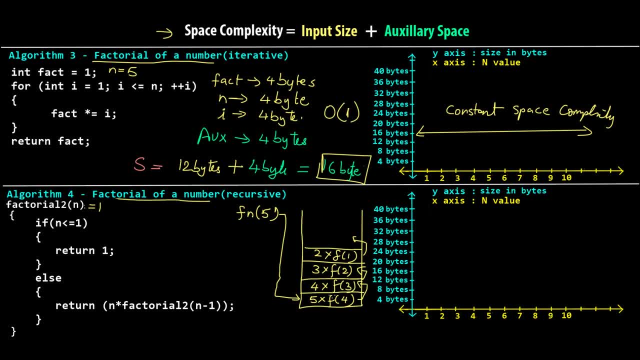 is a system provided memory space which is keeping a track of which function is calling which function. right, And since this is a recursive call, multiple functions, calls are made. So this is basically a memory space. So this might be maybe, let's say, one byte. 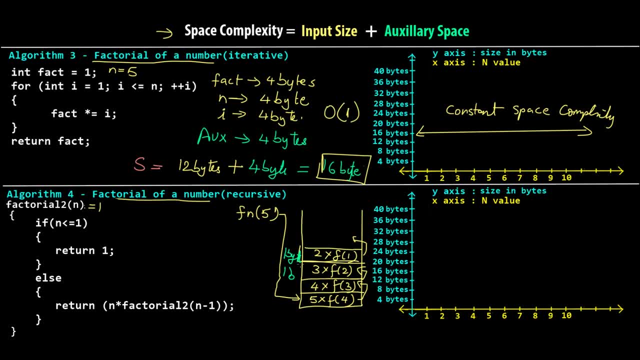 we're just assuming this can be one byte. this can be one byte. it would be a standard size. But as the number of function calls increase, the number of bytes will also increase. That's what I'm trying to see. So when it becomes f of one, we are returning one. So 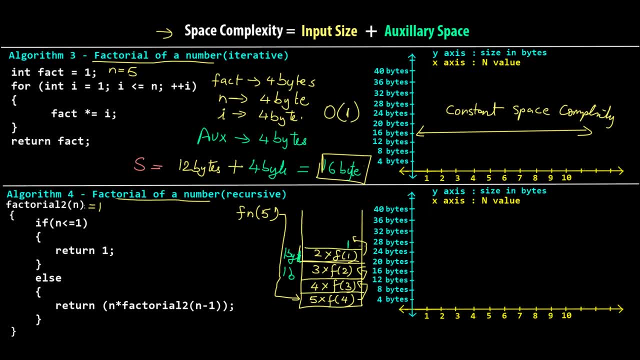 one will be returned over here. So two into one will be returned, And this would go back to the calling function. So f2 had called f1. So two into one is two. So instead of f2, now we have two over here. So I'm going to erase this and we are getting back to 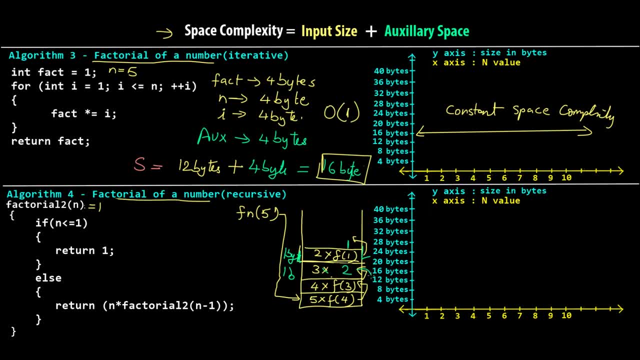 over here. So three into two is six. So six will be returned over here. So if we have six will be returned back over here. which was called by f3. So f3 now becomes six. So four into six becomes 24.. Right, So that would be returned from over here to f4, f4 had called. 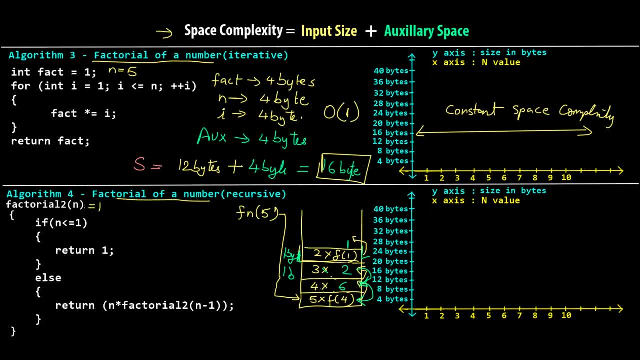 f3, we got the result of f3 as six into 424.. So 24 will be substituted in the place of f4.. Now 24 into five is going to give you 120. And that 120 will be ultimately given over here, returned over here, And we are going to get the result as 120.. Now what just happened? 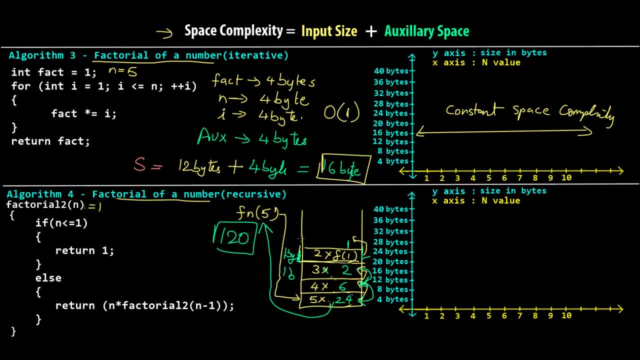 What just happened over here is. I explained to you what is happening behind the scenes. in short, in a quick way: when the algorithm is a recursive type of algorithm And, as you can see, as the number of recursive call increases, the call stack memory also keeps on increasing. 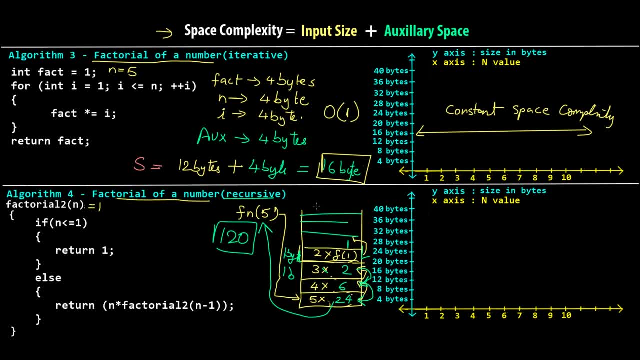 So this is where keeping a track of the space for recursive functions become a little tricky, because those individual intermediate function calls will also have some memory allocations. For example, in one function call what is happening? we are passing n, So n is going. 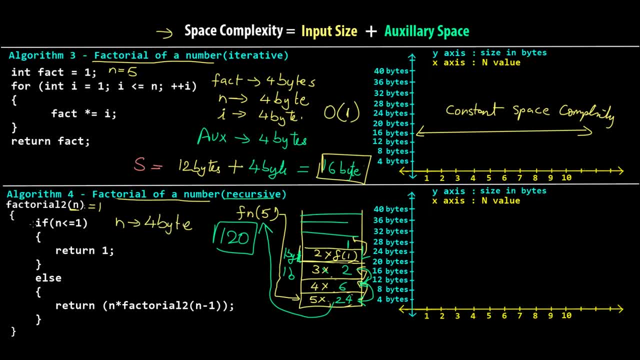 to be four bytes, because n is an integer variable. And then for one function call, we have if statement, we have l statement, So we have auxiliary space for one function call. So the auxiliary space, let's assume, is four bytes, But remember that we are calling. 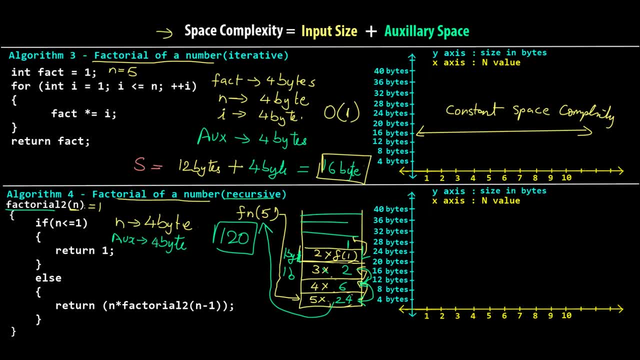 the same function for five times, So four plus four, for one function call, which is equal to eight bytes. And the same function is called five times So eight into five, which becomes 40 bytes. right, You can see there is an exponential growth over here. 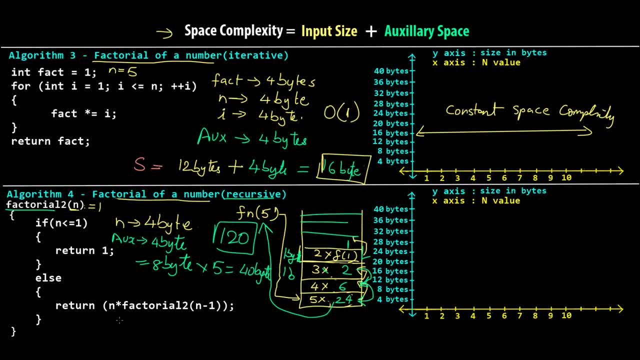 So when you calculate the space complexity for a recursive function, it will be more dependent upon the auxiliary space, that is, this part and not the actual input size. This input size is going to be the constant over here, Because whatever number you enter, that is. 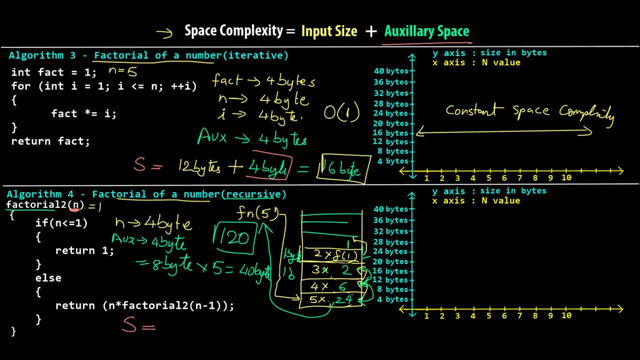 okay, But the number of recursive calls depend on this n, And hence this time the input size is going to be like four bytes only, because that's the size of the integer variable that is going to be stored, But the auxiliary space now becomes variable. The auxiliary space is increasing, which is 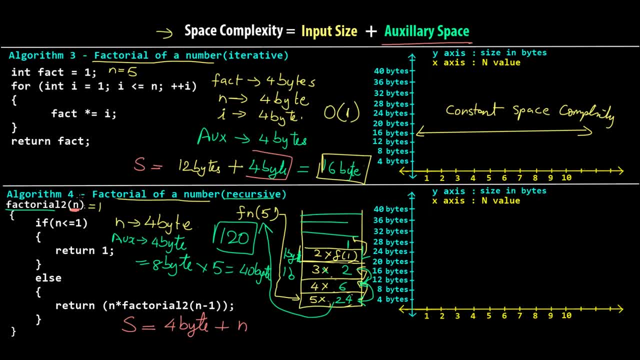 directly proportional to the number that we are passing. So if you're passing five, we are getting five recursive calls. If you're passing six, we are going to get six recursive calls, And then this is going to be n into the bytes for one function call bytes required. 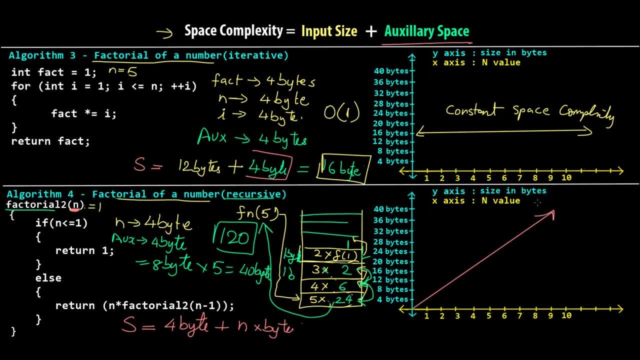 for one function call. So you can see that this can be said as a linear space complexity. But here we are not more interested in the input size When it comes to recursion and recursive functions. we are more interested in the extra space that is required to maintain this call stack and to call the recursive functions and keep. 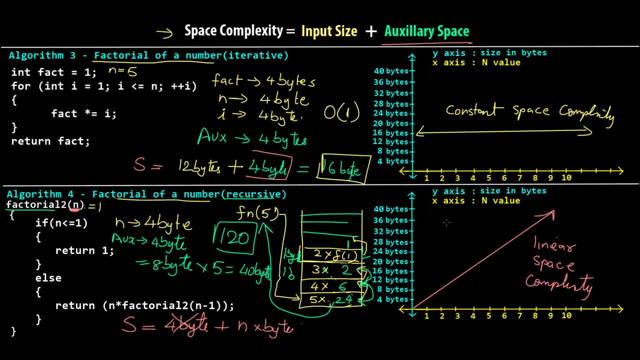 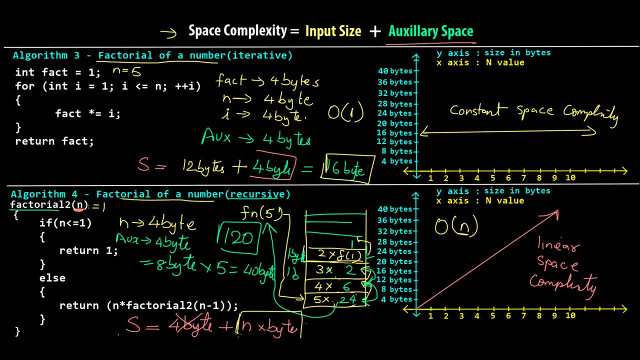 track of them, And that's why here we are going to give this space complexity of O of n. But this O of n is more important or only relevant because of this auxiliary space calculation and not because of the input size. So that's why sometimes only auxiliary space is important. 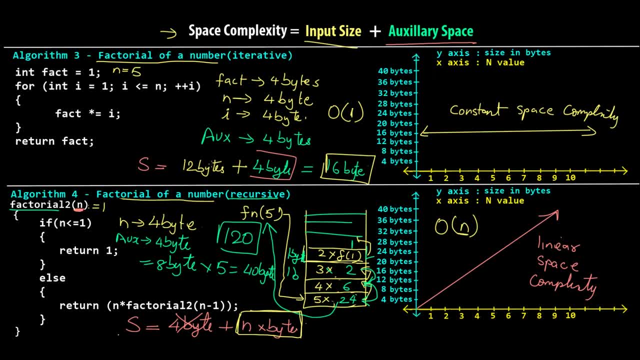 especially when we are giving recursive calls. And if I, if you just go to the next slide, you'll see that this is a recursive space And if you go to the next slide you'll see the sameaken freedom term. you can pull it out if you just Google the space complexity. 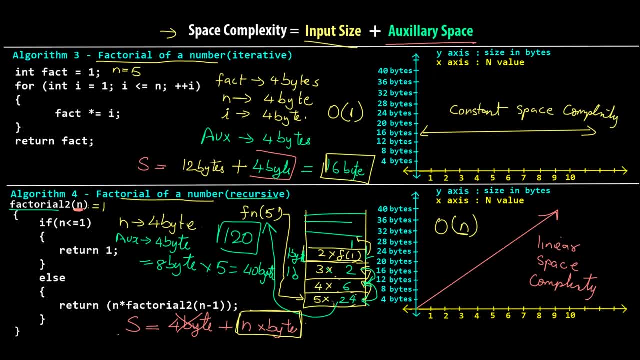 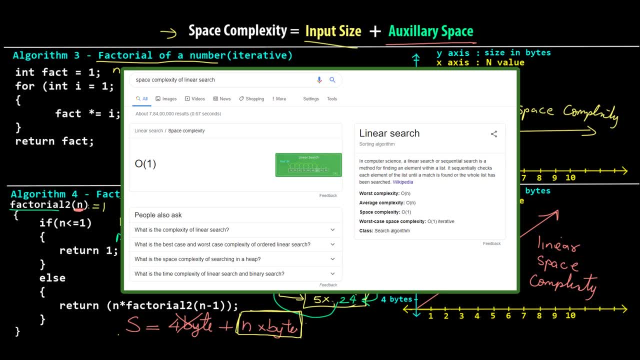 of a sorting algorithm, or you know, let's say, space complexity of a searching algorithm, for example linear search, you'll get the result as O of one. Now, technically, for a search algorithm, for a linear search algorithm, let's say you have- let me just erase this. 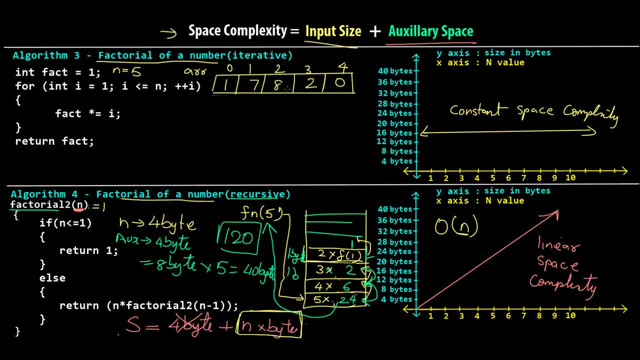 out. So let's say you have an array of size five and you have some integer variables and you want to do a linear search and you want to search for this number zero. So you'll start from one, two, five, eight, two, and then you'll reach to this right. So basically you'll need five iterations. But 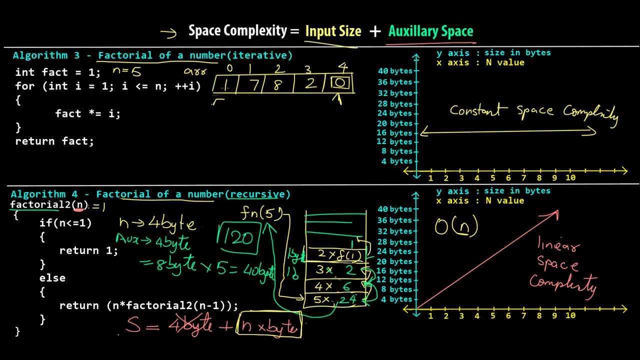 the size of this input array is always going to be same, no matter how many iterations you take. So the space complexity over here is going to be five only. there is no auxiliary space required, right? So if you calculate the space complexity for a linear search, it is going to be the